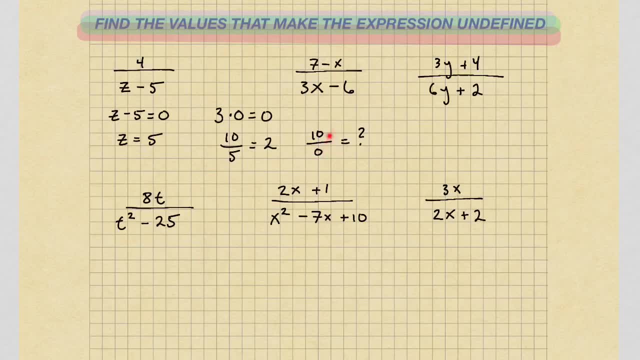 So you're saying some number times 0 equals 10.. Some number times 0 equals 10.. Well, there's no number multiplied by 0 equals 10, because any number times 0 equals 0. So you can't have a 0 in the denominator, That's going to be undefined. 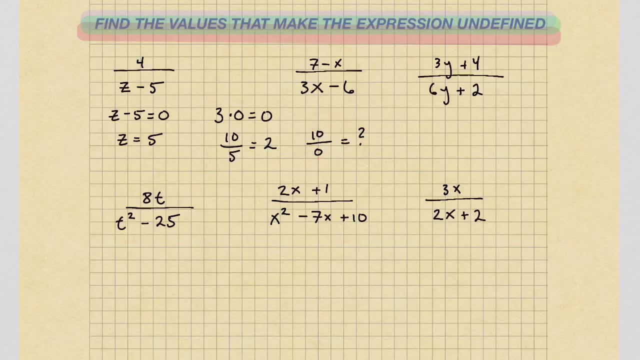 Okay, there's no number here that's going to make this true. Okay, so what we do is we just set these denominators equal to 0.. And that's where this expression is undefined. So it's very simple: We just go through these expressions and set the denominators equal to 0.. 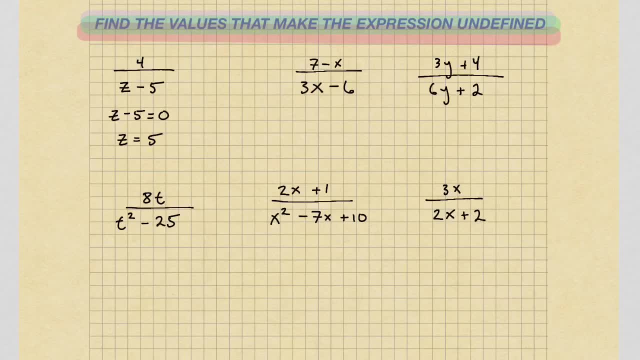 And then find out where that's true. So for this next one, we have: 3x minus 6 equals 0. Okay, adding 6 to both sides, we get 3x equals 6.. Dividing by 3,, we get x equals 2.. 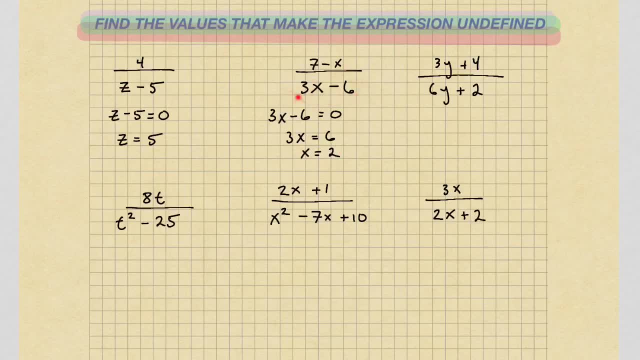 So if I were to plug in this number 2 into this expression, 3 times 2 is 6 minus 6 is 0.. So x equals 2 is where this expression is undefined. Okay, very simple, We just take the denominator and set it equal to 0.. 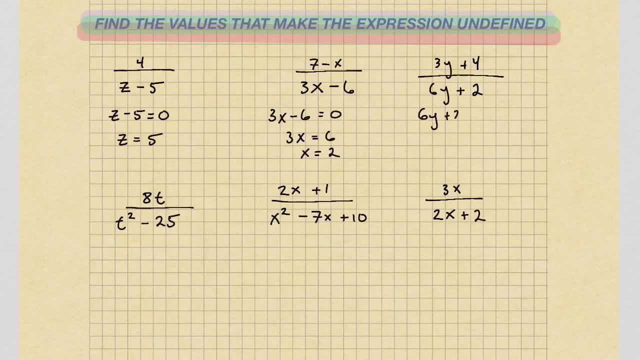 Okay, so for the next one, we have 6y plus 2 equals 0. Subtracting 2 from both sides, we have 6y equals negative 2.. Dividing by 6, we have y equals negative 2 over 6.. 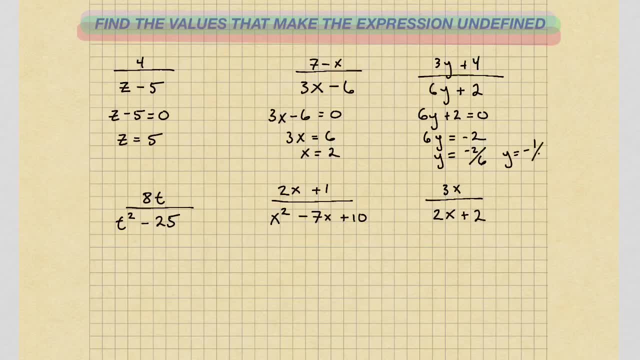 Or y, equals negative 1 over 6.. Negative 1 third. So if I plug in this number, negative 1 third- if I plug it in here to the denominator, it's going to be equal to 0, therefore undefined. Okay, next problem: we have 8t divided by t, squared minus 25.. 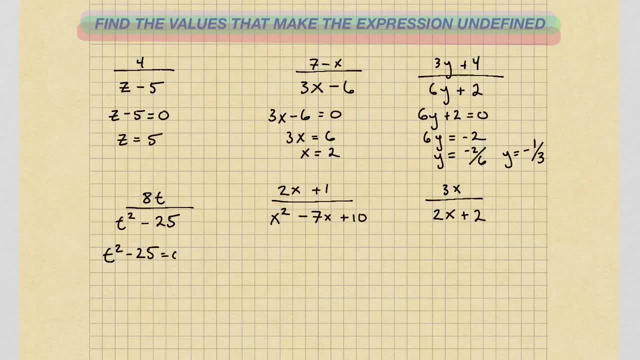 So we're going to say t squared minus 25 equals 0.. And t squared equals 25. by adding 25 to both sides, Now, taking the square root, we have t equals plus or minus 5.. Okay, remember, if we introduce a square root to both sides, 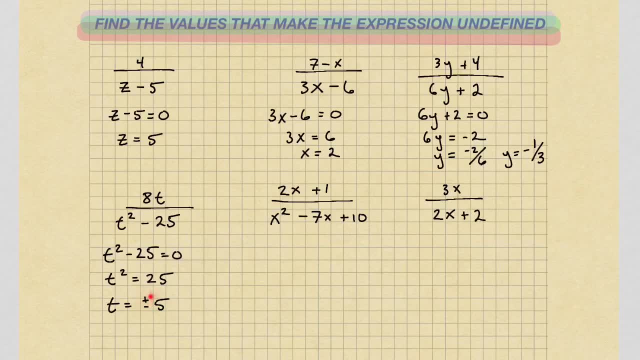 we have to include both positive and negative. Okay, we introduced the square root here. Okay, that's the step that we introduced the square root, from this step to this step. So we have to include both positive and negative numbers. So what that means is, you know, you have negative 5 squared. 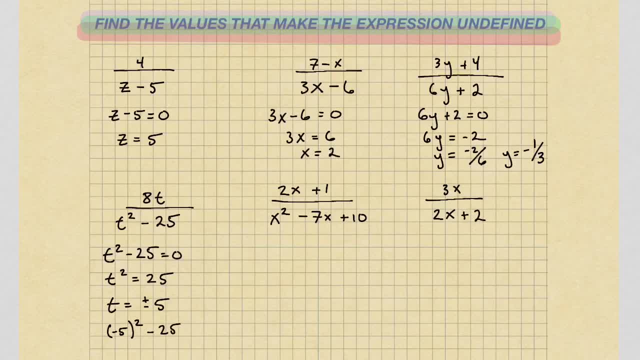 plug it in: negative: 5 for t minus 25. That gives you 25 minus 25.. That equals 0.. Same with positive 5.. 5 squared minus 25. That also equals 0.. So keep in mind if you introduce a square root. 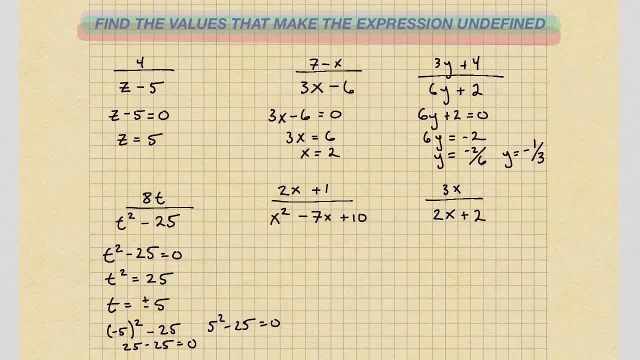 that you have to include both positive and negative values. Okay, next one: we have x squared minus 7x. 7x plus 10 equals 0.. Okay, what we're going to do is we're going to factor this trinomial here. 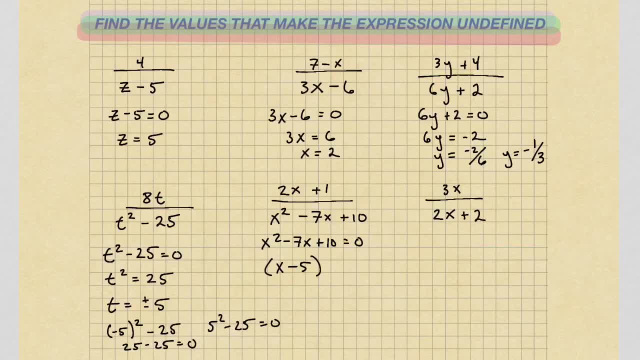 And we have x minus 5 and x minus 2 equals 0.. So we know that x equals 5 or x equals 2 will make that come true, So we plug in a 5.. Then we have 5 minus 5 equals 0. 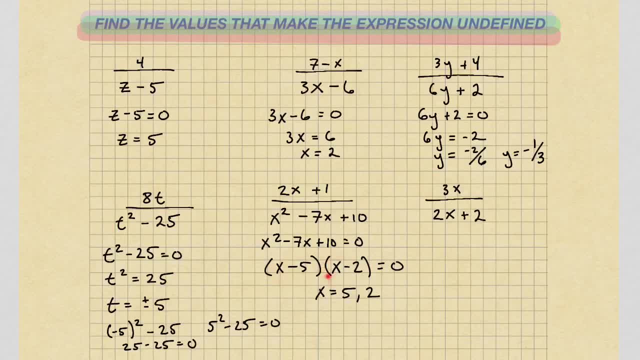 0 times whatever's left. 0 times anything is 0.. Same with the number 2.. We plug in the number 2.. We have 2 minus 2.. That means this expression. here this turns to 0.. And 0 times anything is 0.. 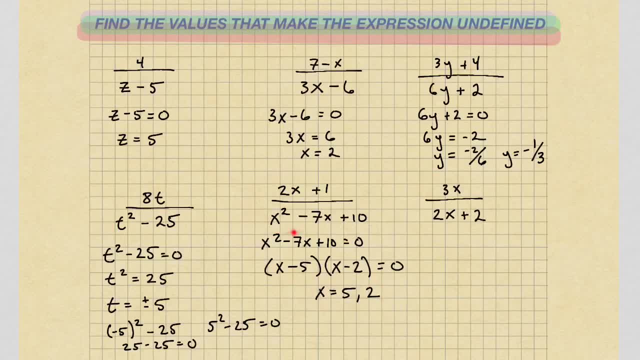 So here is your two values that make this expression equal, undefined. Okay, the last one. here we got 2x plus 2 equals 0.. 2x equals negative, 2.. x equals negative 2 over 2.. That means x equals negative 1.. 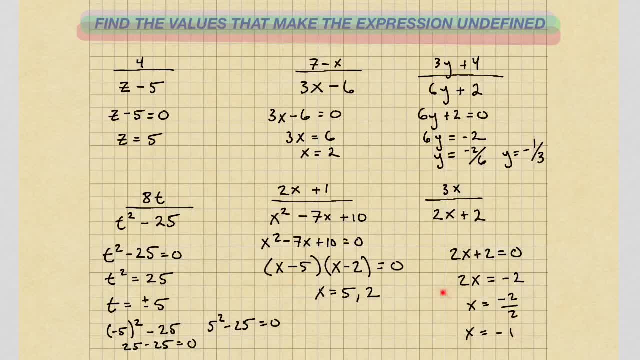 So if I plug in the value of negative 1,, then this denominator is going to go to 0,, leaving it undefined. Okay, pretty simple. Just keep in mind why you can't have a 0 in the denominator. The denominator goes back to your arithmetic rules.